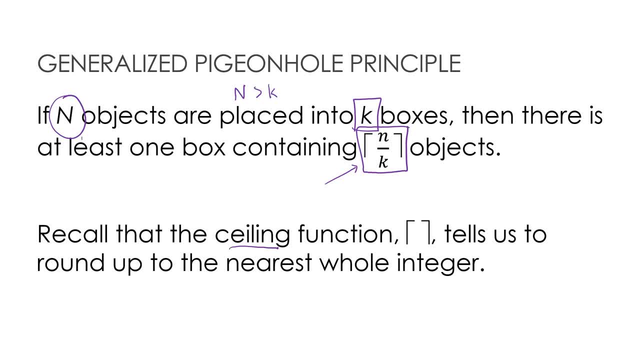 us to round up to the nearest whole integer. So for instance, I had 27 English words and divided by 26 letters in the English alphabet, This number is a little bit greater than one, and this ceiling function says: round that to two. So we know that at least one box contains. 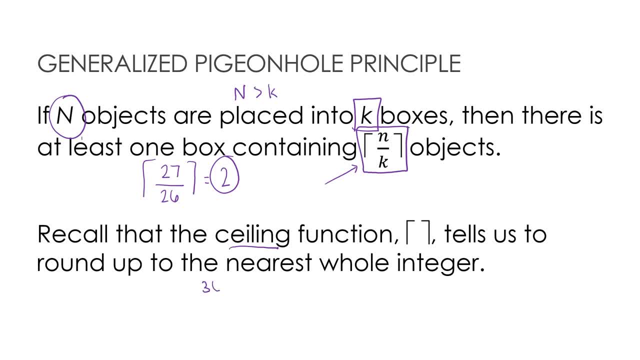 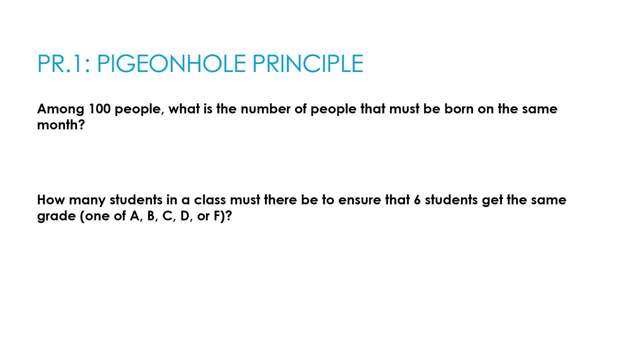 two objects. If I had my 367 people in a room divided by 365, again, this value is greater than one, Greater than one says round up to two. So at least two people in that room must have the same birthday. So here are a couple of questions for you to try Again. these are: 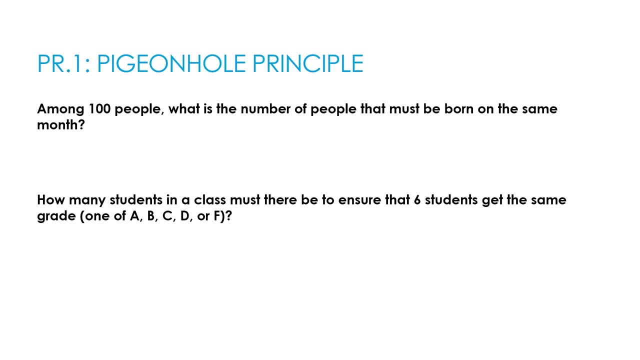 pretty straightforward, easy examples of the pigeonhole principle, and then we're going to get into some that are a little bit more complicated. But I'd like you to press pause and try both of these questions first and then press play to see how you did. 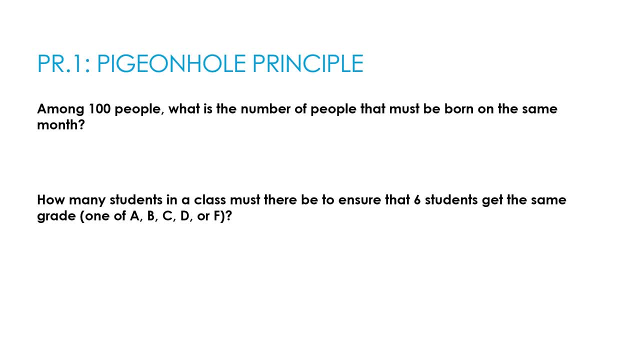 So again, among the first 100 people, what is the number of people that must be born in the same month? So if it's in the same month, we're talking about the ceiling function, which is the number of people that must be born in the same month. So if it's in the same month, 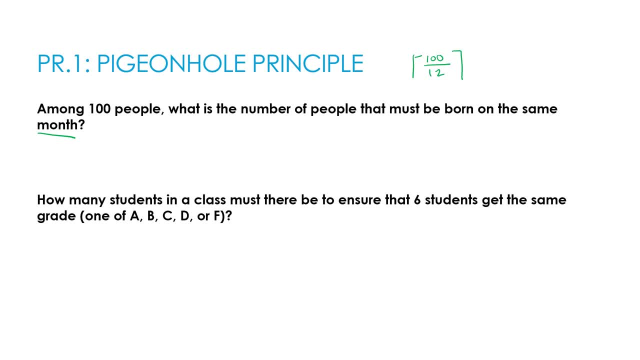 we're talking about the ceiling function, which is the number of people that must be born in the same month, Of 100 divided by 12.. That's how I would go about solving this. So 100 divided by 12, rounded up to the nearest whole integer is nine. So there must be at least nine born on the same. 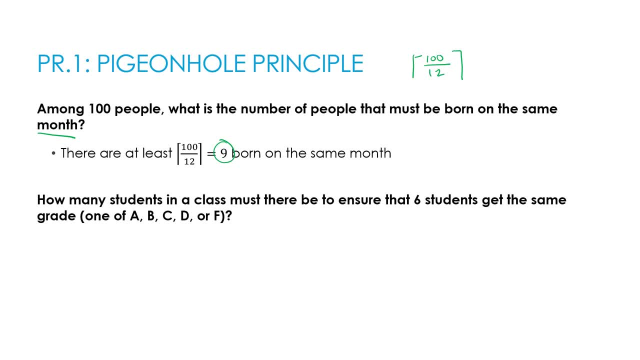 month? How many students in class must there be to ensure that six students get the same grade? And, of course, there are five grades. Now, this one's a little bit different, because we're still using this pigeonhole principle and the ceiling function. 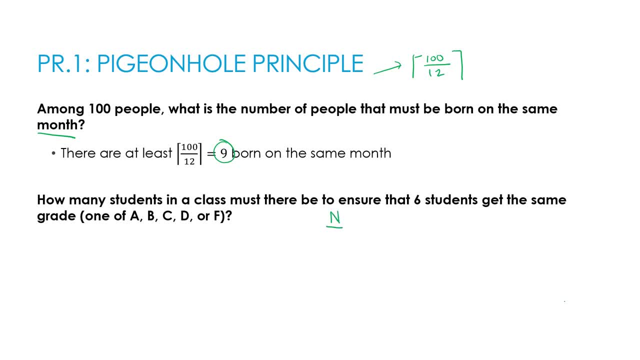 but I don't know n. So I'm saying n divided by the five grades has to be equal to six. That's essentially what I'm solving for. So it's not as easy as just saying: well, five times six is 30.. 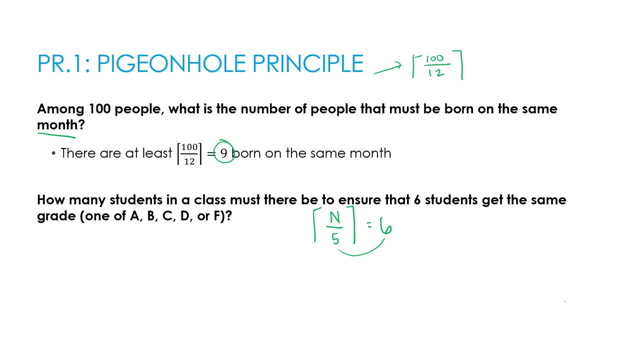 So it's got to be 30. Because, remember, it's anything that rounds up. So if I say, said n was 25, well, 25 divided by five is exactly five, ceiling function or no. So the lowest number must be 26.. 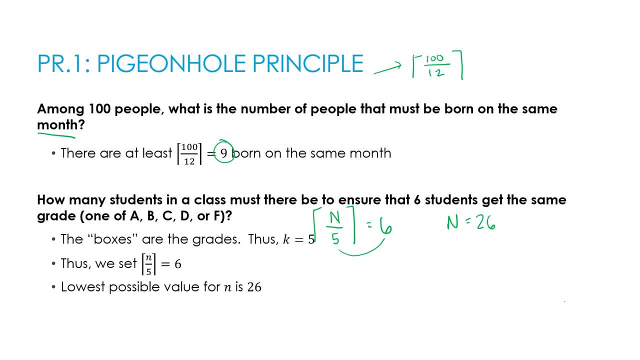 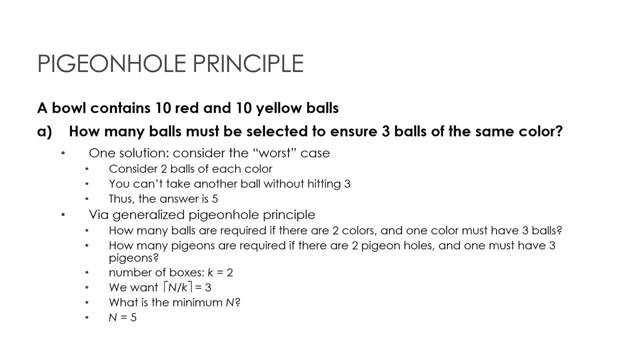 So the lowest possible value must be that n is 26.. Because 26 or more would mean that six students would get the same grade on whatever assessment they're taking. Before I set you loose on a couple of questions that will maybe stretch your brain a little bit, 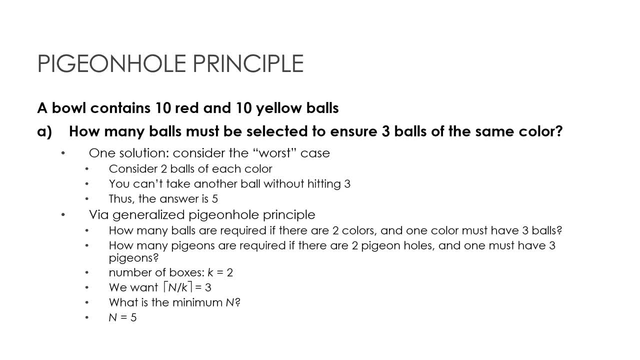 I want to go through a little bit of math with you. So let's say I have a bowl, I've got 10 red and 11 yellow balls in the bowl. So 20 balls, 10 red, 10 yellow. A says how many balls must be selected to ensure three balls. 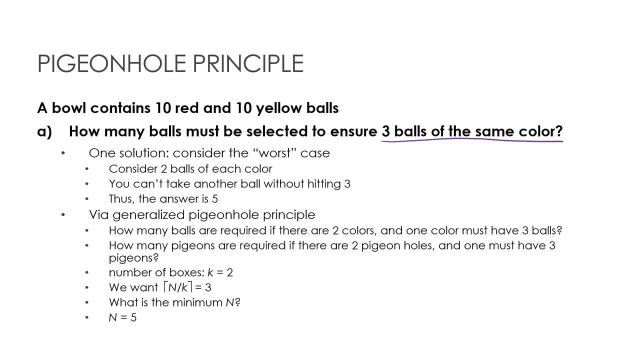 of the same color. So I can look at it two ways. I can say: let's look at the worst case scenario, which means the most number, So to get three balls of the same color, I could say my first one was yellow. 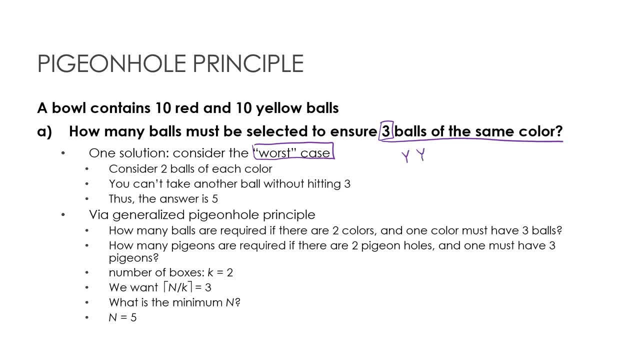 my second one was yellow. I don't want to pick another yellow yet because that's not worst case. that's best case. then I get a red, then I get a red. at this point I'm stuck because whatever I pull out next, yellow or red, that's gonna give me. 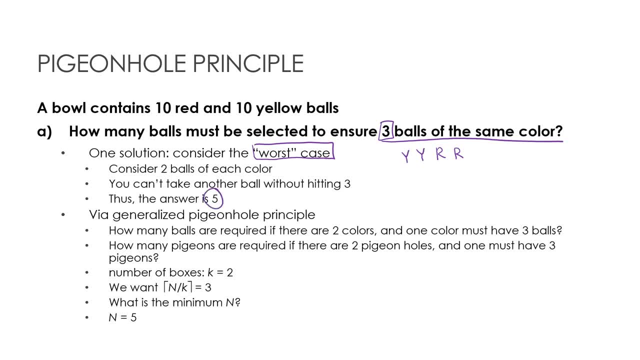 three of the same color. so the answer is five. so I can do it without using the ceiling function. or in this case, I can still look at the ceiling function and say there's two colors, which is essentially two boxes. so I'm saying n divided by two has to be three. so what does n have to be? well, four divided by. 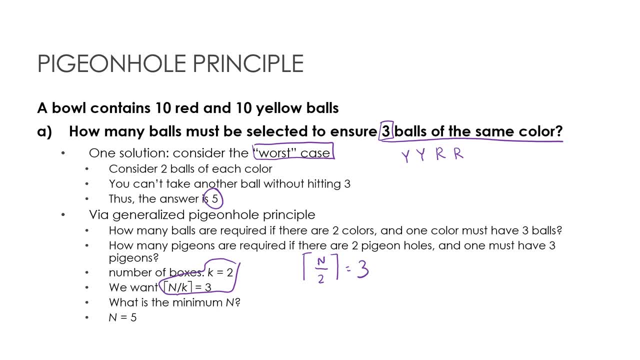 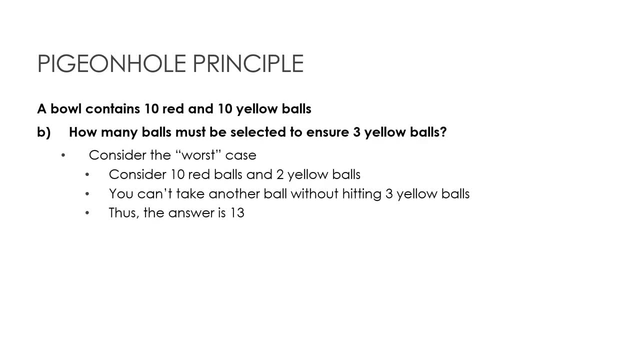 two would give me two. five divided by two would give me two point five, which rounds up to three. so n must be five. now this one not quite as straightforward, because now I can't just rely on the ceiling function. we're not just saying: ensure three of the same color, we're specifying three. 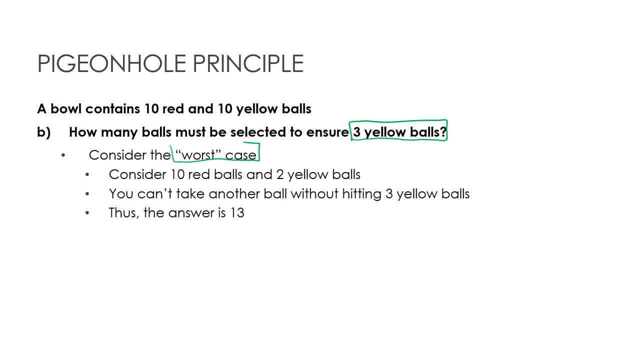 yellow balls. so again I'm gonna look at the worst-case scenario, or what's the most number. well, it could be that my first ten balls are all reds, and then I get a yellow, and then I get a yellow, and now I'm stuck because now there's no. 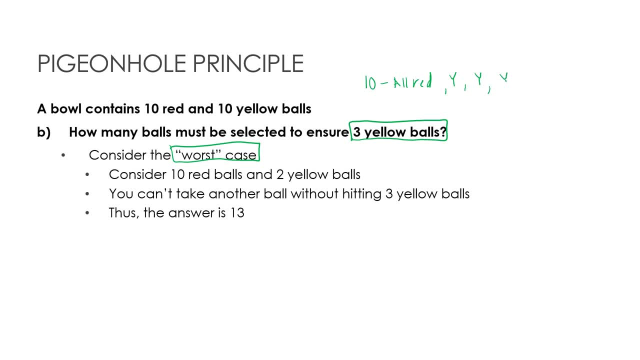 more reds to take out, and the only thing left is a yellow, and so it must be 10 plus one yellow. and then I'm stuck, because now there's no more reds to take out and the only thing left is a yellow, and so it must be ten plus one. 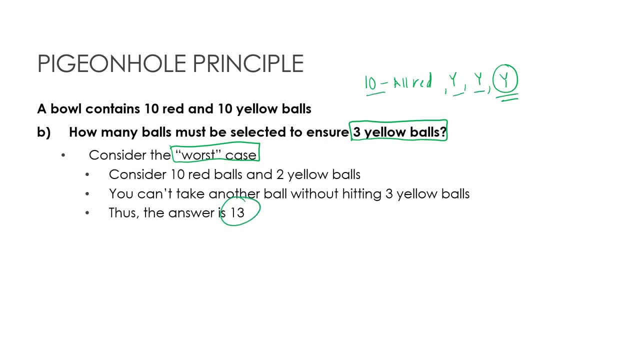 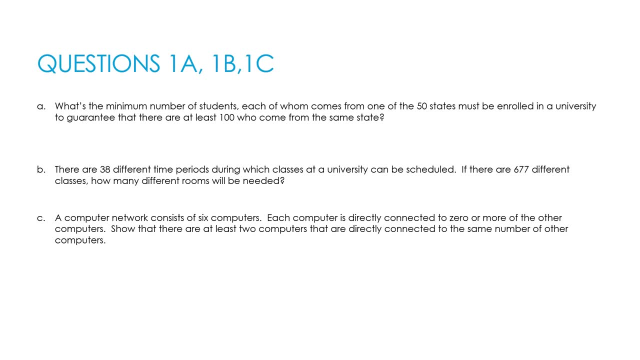 plus one plus one or 13 balls. So that's the worst case scenario. The next three slides all contain questions that I'd really like you to struggle with a little bit before you go through the answers with me. So what I would suggest doing if you are actually enrolled in my class and not just watching this video. 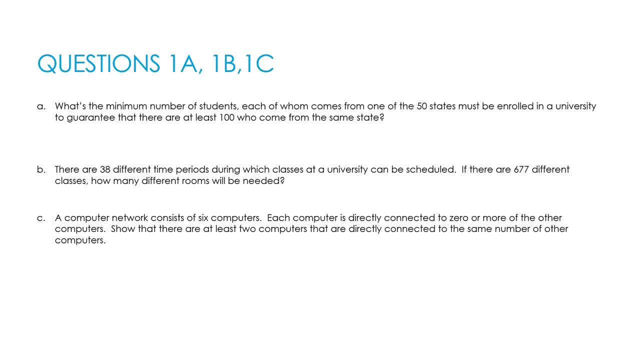 for fun is actually trying these questions on your own, collaborating with your classmates in the team's environment, to try to come up with the answers to these, before you just press play and see what the answers are, Because it's much more beneficial for you as a student to actually have tried. 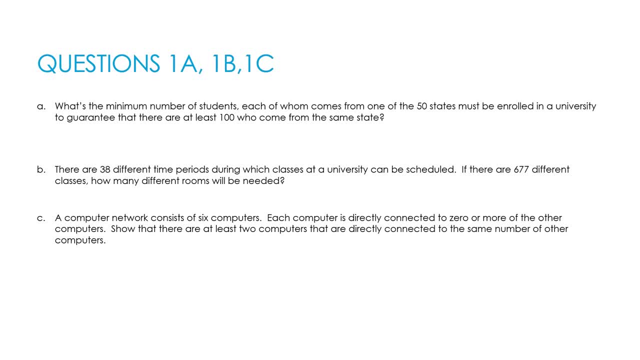 these and to struggle with them a little bit before you just find out what the answer is. So here's the first three questions. Again, I would press pause. read the questions, try each one, work with other people. When you're all done, then you can watch the video to see. 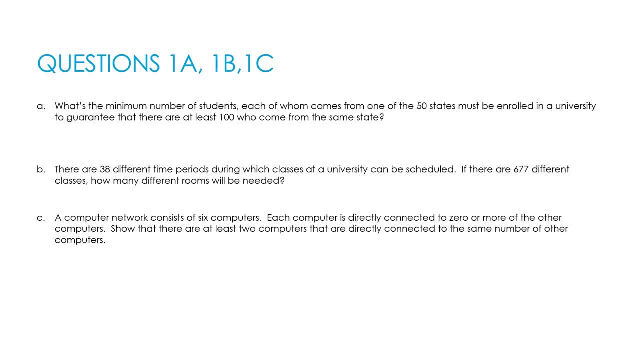 what the answers are. So for the first one, what is the minimum number of students, each of whom comes from one of the 50 states, must be enrolled in the university to guarantee there are at least 100 who come from the same state. So again, we're saying that that number must be 100 and they're asking: 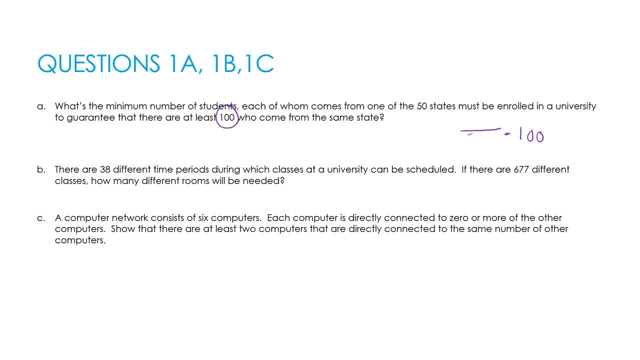 for what is n for this to be true? So we've kind of looked at these before, but we didn't really talk about what's the math involved in how to get there. So what I can really do is I can take this number and subtract one, So instead of 50, 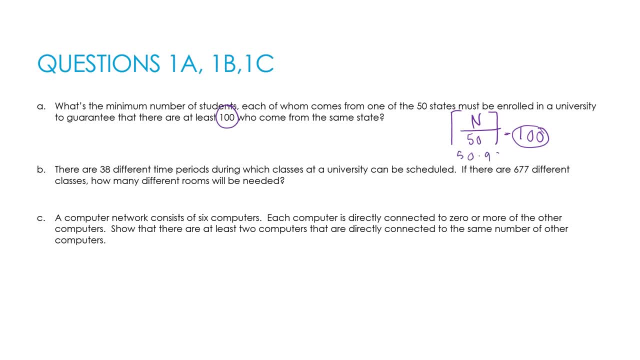 times 100. take 50 times 99, because 50 times 99 would give me 99. Here and then add 1 to that. so 50 times 99 plus 1 is 4951.. That is the minimum number of students to guarantee at least 100 come from the same state. Part B: 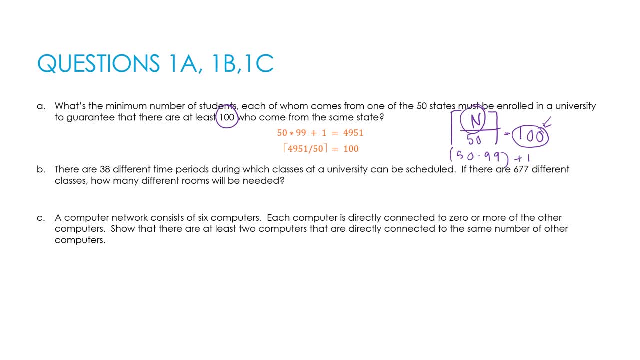 There are 38 different time periods during which classes at a university can be scheduled and 677 different classes. How many rooms will be needed? This one is this one's real, straightforward ceiling function: 677 divided by 38, and that gives us 18. 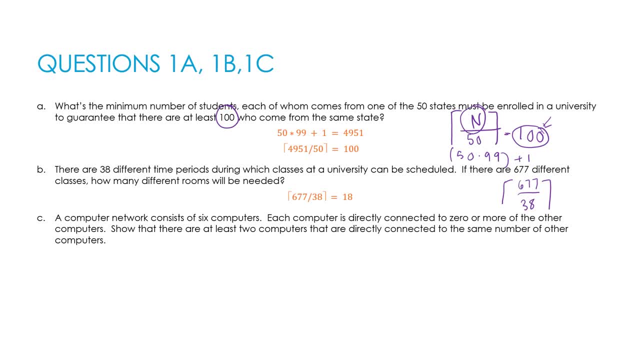 last one computer network consists of six computers. so we have six computers. each computer is directly connected to zero or more of the other computers. so again we think: what are the number of pigeons, what are the number of boxes? well, we know that I have six things. 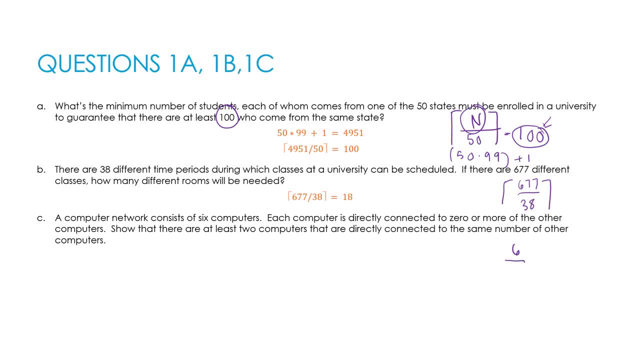 and the question is: what's the number of connections? well, if it's connected to the other computers, obviously we're not gonna have a computer connected to itself. so five is the most number of connections, because we could have one connection to connection, three, connection for connection, five connections. so 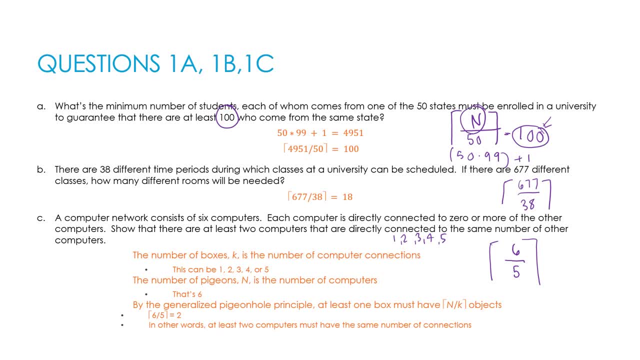 essentially, I'm taking the ceiling function of six divided by five, which is two if I round up, that's the ceiling function. so basically, I have just shown- that's what I'm asked to do- that there are at least two computers that are directly connected to the same number of other computers. 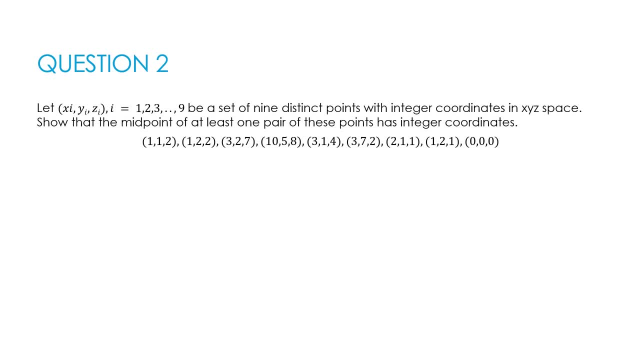 question two, and yes, these get harder as we go. question two: we have a set of nine distinct points with integer coordinates and XYZ space, so three-dimensional show that the midpoint of at least one pair of these points has integer coordinates. now, of course, I couldn't go through and find the midpoint of all of these points. 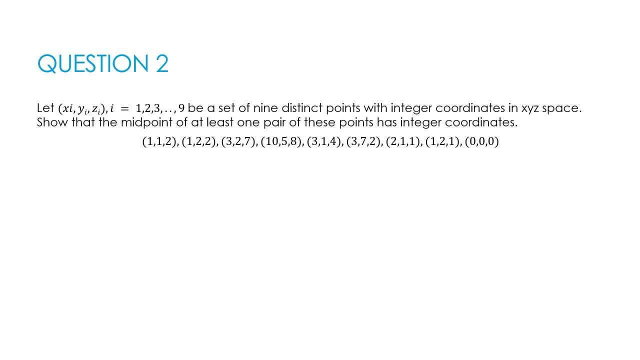 but let's go about this in a mathematical way instead of a plug-and-chug kind of way. what do we know about integer coordinates? actually, if let's start with, what do we know about the midpoint? well, the midpoint says: in order to find the midpoint, we need to take the x-valve and y-to-Z values. 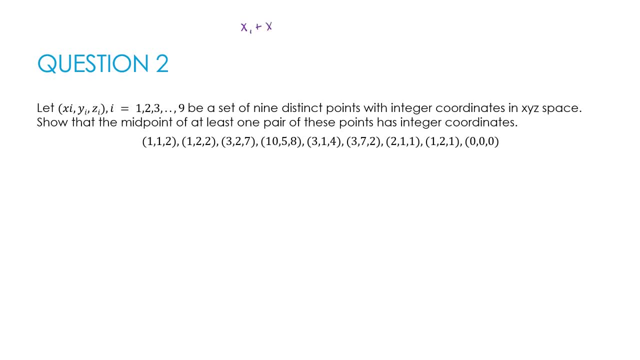 value of the first one plus the x value of the second one and divide it by two. That's what the midpoint formula says. So if I'm doing this for x's and y's and z's, oops, z1 plus z2 divided by: 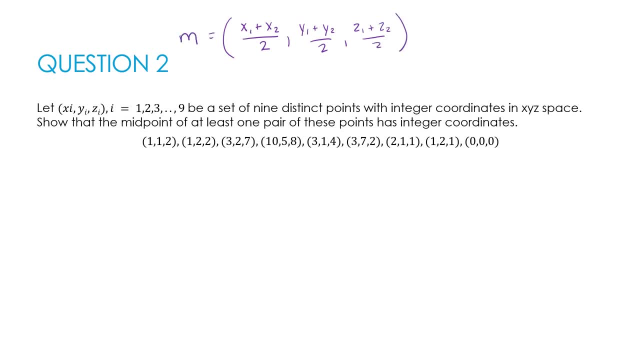 two. that's my midpoint. Notice, all of these are divided by two. So essentially, what I'm saying is: the sum has to be even. Well, why does that matter? Well, it matters because if I take an odd number plus an odd number, what do I get? I get an even number. If I take an even number, 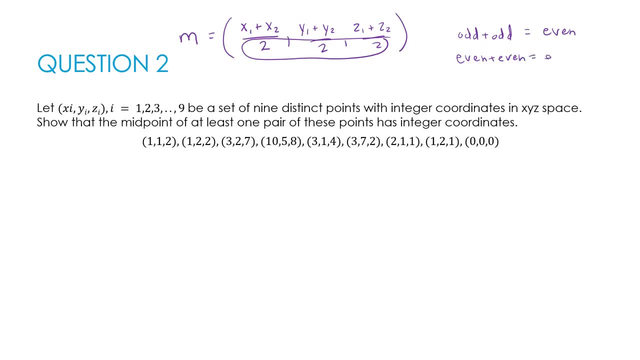 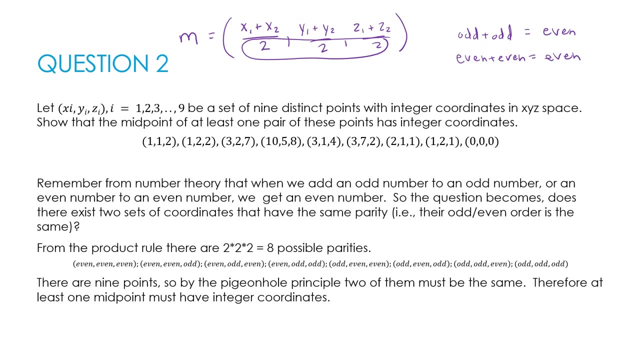 plus an even number. what do I get? I get an even number. So that's how I'm going to go about this question. What I want to do is I want to look at the possible parity. So parity just means if it's even or if it's odd. So from the product rule we've got an even or an. 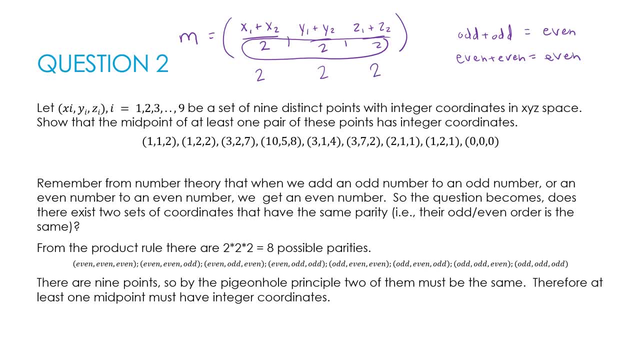 odd here, an even or an odd here, an even or an odd here. Two times two times two is eight. So there's eight different possibilities, And now I've listed them here for you. but that's not necessary. So essentially I'm saying it could be an even number comma, an even number comma. 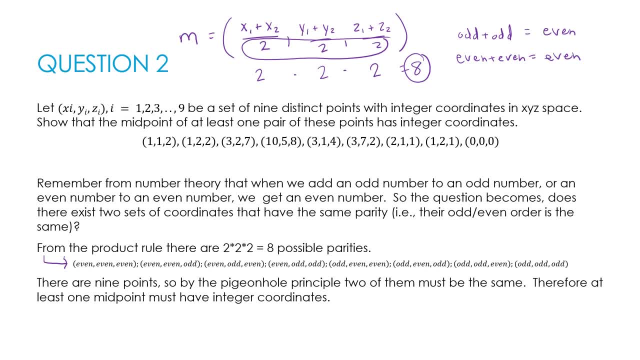 an even number, Or an even even odd, et cetera, et cetera, et cetera, because these are ordered triples. So eight is essentially the number of boxes. Well, how many points do I have? They gave me nine, So 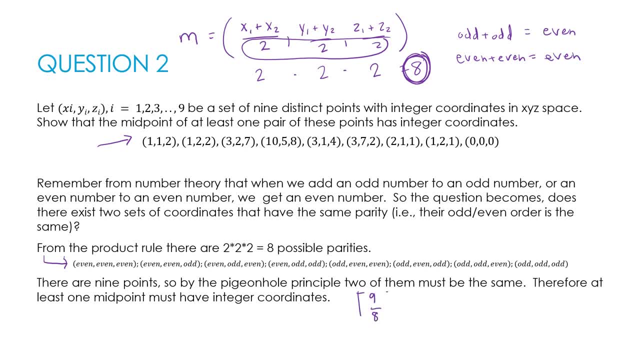 essentially, I'm saying nine divided by eight, which of course means two of them must be the same. All right, let's take a look at this last question. During a month with 30 days, a basis of 10 days is equivalent to the sum of the number of boxes. If there is a non-elemental 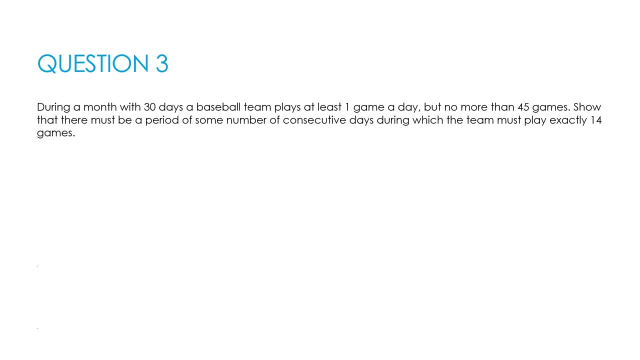 team plays at least one game a day, but no more than 45 games. so there must be a period of some number of consecutive days during which the team must play exactly 14 games. so again, I encourage you to press pause to try this question all by yourself or with your classmates, before you just press play to see the 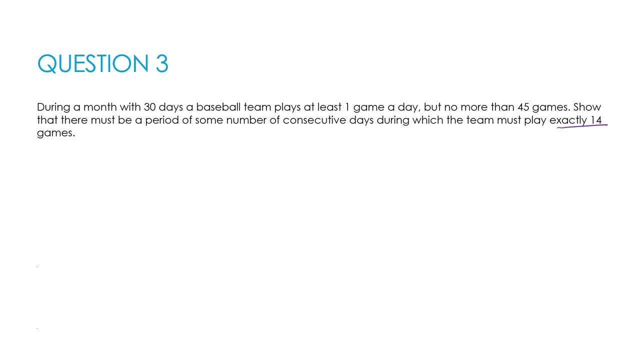 answer, but this one will stretch your brain a little bit. let's start by saying we know that, because they play at least one game per day, but no more than 45 games, that our number of games that they play each day is going to increase. so I'm never going to have two days in a row where I've played the same number of. 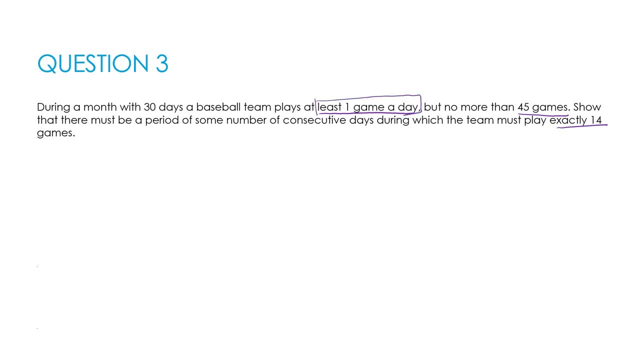 games, because they're playing at least one game a day, which means if the first day I play one and the second day I play one, then the second day I've actually played two, one the day before and one that day. So you get the idea. So what I'm going to do is 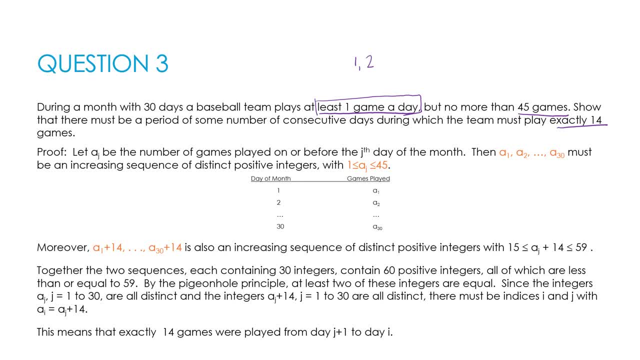 I'm going to let a sub j equal the number of games they've played up to that point, up to the jth day of the month. So a sub j is going to be the number of games played on or before the jth day. Then my series of numbers must be increasing, which we know because it's 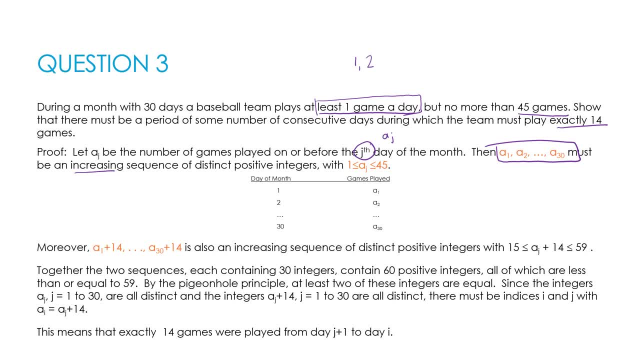 increasing by at least one every day, and they're going to be distinct, which means I'm never going to have the same number twice, because even if I just play one a day, that number is different each time that I do it. So essentially, what I'm saying is that a sub j 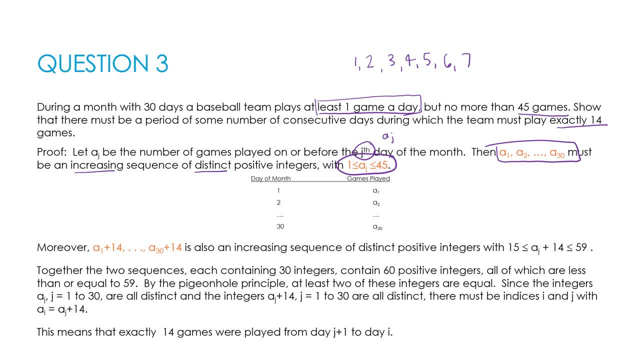 is going to be. the number of games they've played up to that point, up to the jth day of the month, Must fall between 1 and 45.. 1 is the minimum because I'm going to play at least one game on. 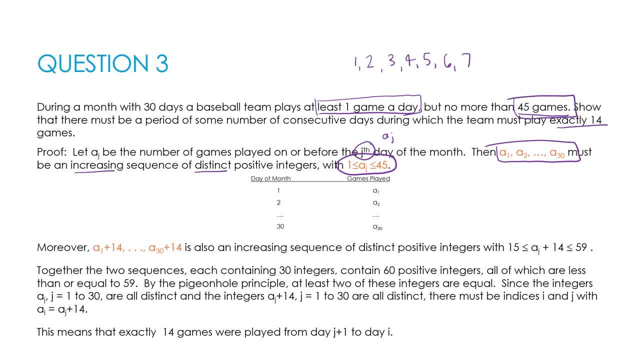 the first day, but I can't do more than 45, so 45 is my max Now. hopefully that has made sense so far. Now let's take this guy and just for fun, because we're dealing with 14 games, let's take. 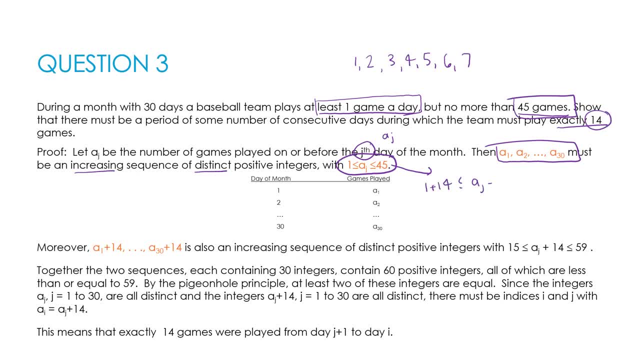 1 plus 14, a sub j plus 14, and 45 plus 14.. What does that give me? That gives me: 15 is less than or equal to a sub j plus 14 is less than or equal to 59.. Do you agree that that is still true? Sure, because I just did a.